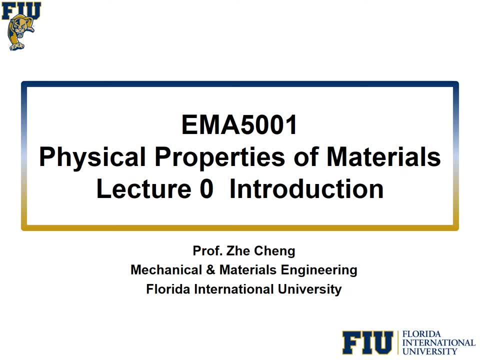 hi everyone, my name is Li Cheng and I'll be your instructor for this class, EMA 5001. the official name for this course will be so-called physical properties of materials, but in my opinion this is a so-called misnomer. our actual course name should be called something like kinetics and phase transformation again. 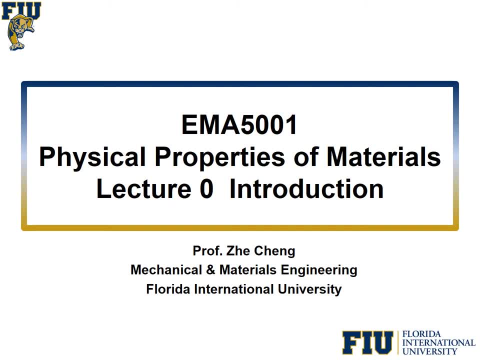 kinetics, which means how fast stuff or things happen, and phase transformation is the transformation going from one phase to another phase. what does phase mean? well, you probably learned in before in your physical chemistry or material engineering course. phase is a portion within the system that is uniform in its chemical and the physical. 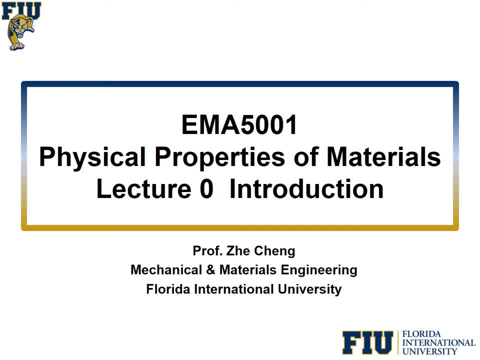 characteristics- chemical and physical characteristics. that's a phase going from one phase to another phase. that's phase transformation. so that's what this course will be about. kinetics: how fast going from one phase to another phase. how fast does the so-called diffusion process happen? okay, and the phase transformation: how would it happen from one phase to another? 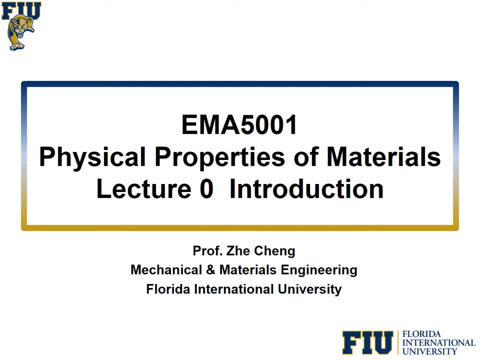 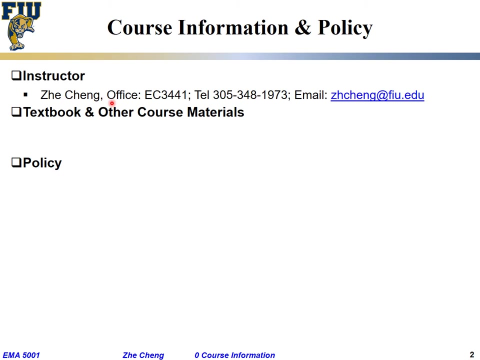 phase. that's what this course is about. okay, and today will be our lecture zero. I call it a lecture zero introduction. okay, first about myself, Li Chen, and my office is at engineering center 3441. you probably saw my door is open most of the time. okay, my phone number is here you. 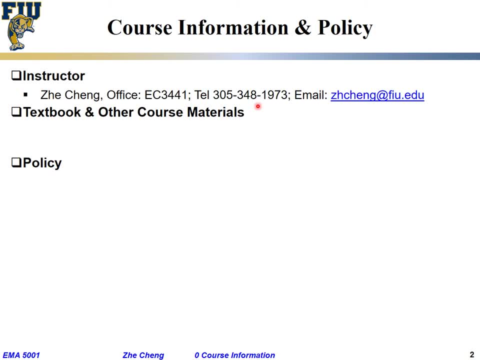 are welcome to call my office phone. you are welcome to call my office phone before you start buying. you can call me three times. do you all make sense to me by? you can call me. okay, you're in office. can i stop by? if i'm busy i would say no, but the most 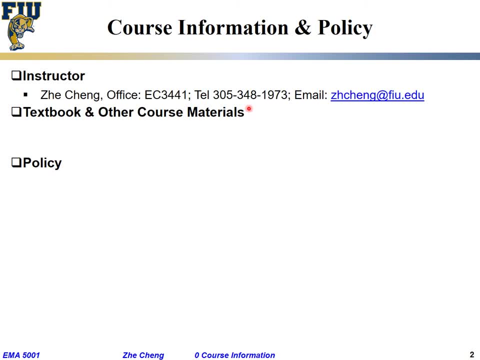 case, i'm available, okay, and you are also welcome to send emails to me. i'm pretty fast, as some of you know, in replying to emails. okay, and the textbook with that, the phase transformation in metals and alloys by da potter. we're using the third edition published in 2008. 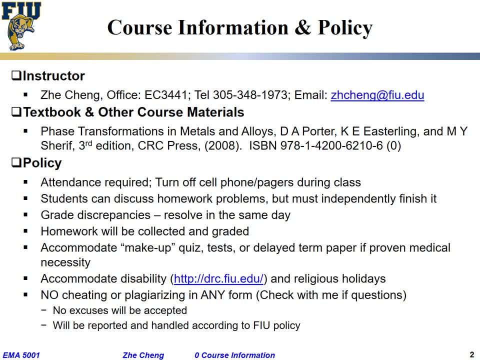 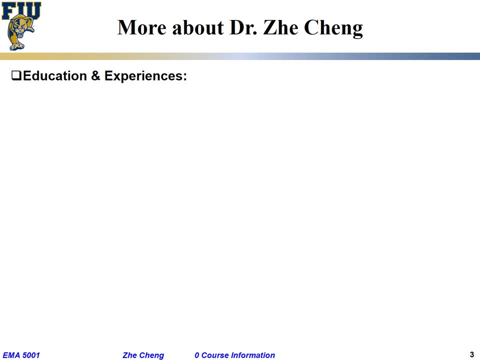 okay, course policy. i'm not going to read it, but it's pretty obvious stuff for graduate students. a little bit about myself for those of you who do not know me. i got my bachelor's in china, beijing, china, and then i came to the united states for phd. 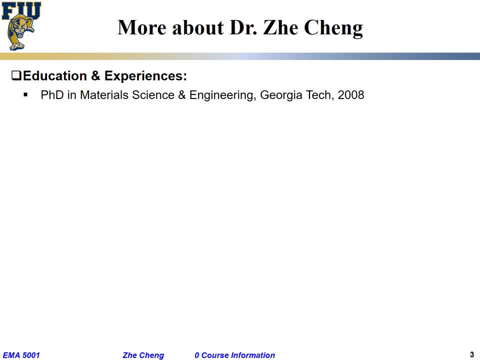 actually master and phd. i got my phd in material science and engineering from georgia tech in 2008- 10 years, 11 years now, 11 years ago, time flies. and then, after i graduated, i went to work in a company called called dupont. now dupont is part of so-called dao dupont because those two companies merged. 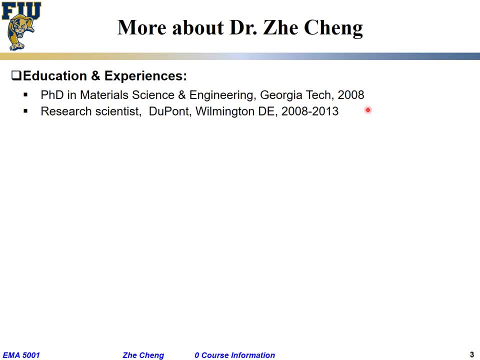 it was one of the major chemical material company in the world. okay, i worked over there in the so-called central research division from 2008 to 2013 for five years as an industrial research scientist. okay, and then in 2013, after i worked for five years, 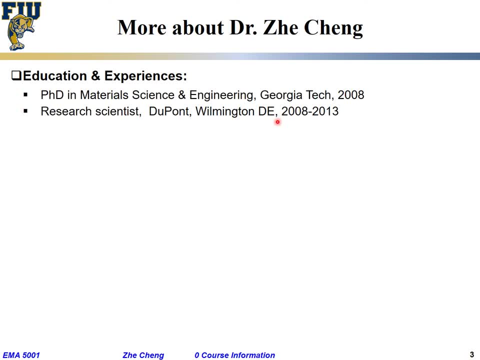 i got. i have to say i got lucky and got the opportunity to return to academia, which is fiu okay, and since then i was and i have been the assistant professor of the department in our mechanical material engineering department- okay, and our research group website is at. a for apple, c for charliefiu dot edu. 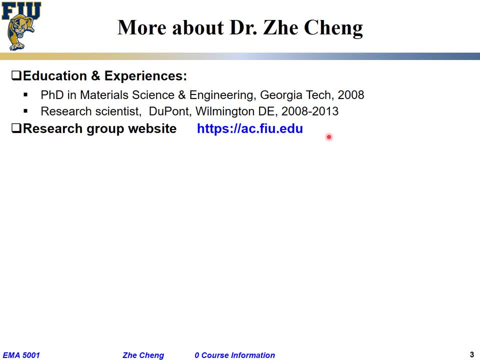 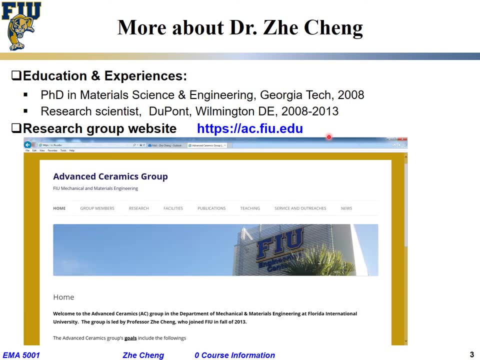 you can go to this website and check for information related to the things that i do, our my research group does. this is just a screen capture. we call ourselves advanced steth i'am Meetings았 group, which means hopefully we don't miss the lessons. also, we'd be really incredibly very proud to have our um. our research group is at the ak for apple for charliefiuedu and our research group is at Ac for apple for charlie Process is for you to find this for us in a little bit. we'd like to remind you that we are notel, because the things here on the slideี่ arefulness, fiction and a whole notel. I can't really help you. 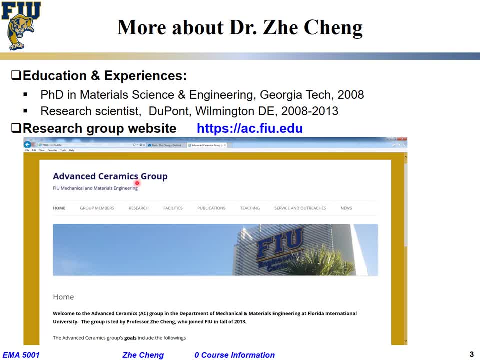 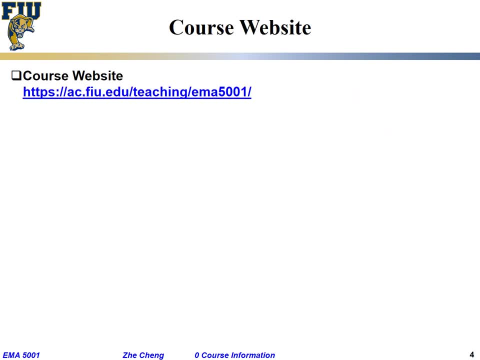 we're working on ceramics and hopefully advanced. that's a just a catchphrase. okay, and, as I mentioned, we have our course website. at our group website. if you click the link in teaching you will find the course and the web address is again given here. and when you check out the course website, you are going to see 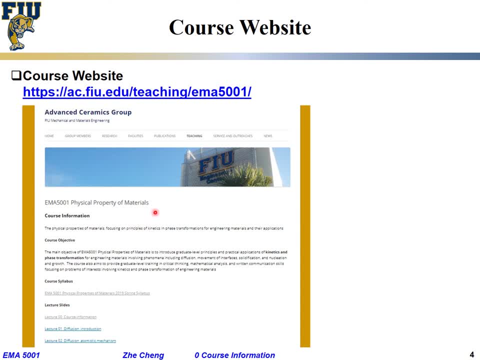 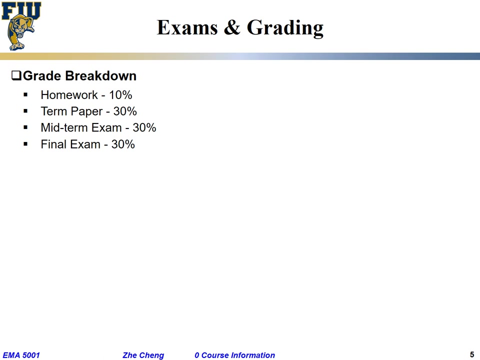 okay, physical property of material and in that you find also the information for this course, as I said, syllabus, and all the lecture slides in PDF format and hopefully in future I'm going to add the video or audio content. okay, you are going to find all the information for this course in PDF format and all the 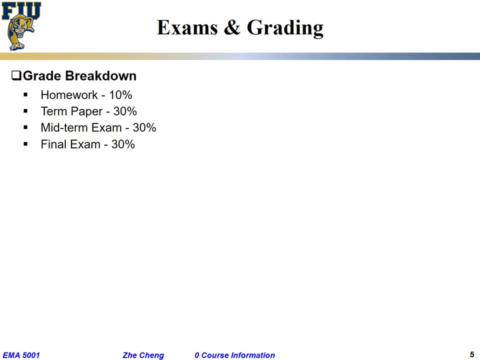 something of course you care would be exams and greetings. the grade breakdown, as you see here we have 10% coming from homework, 30% come from a term paper and I'll explain later. another 30% come from midterm exam, typically before the spring break week. okay, 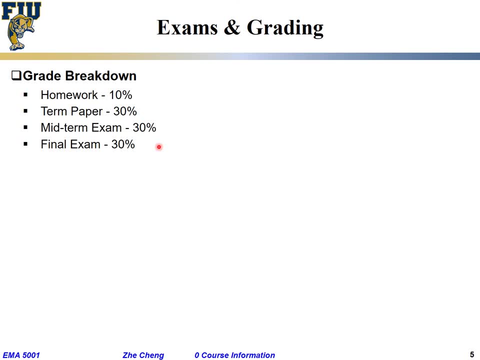 and final exam contribute to the rest of the 30%. okay, under the final grade conversion, I have it here to get A, to get B, to get C, to get D. and keep in mind that I do give low grades. I do give low grades. sometimes I give B and then I 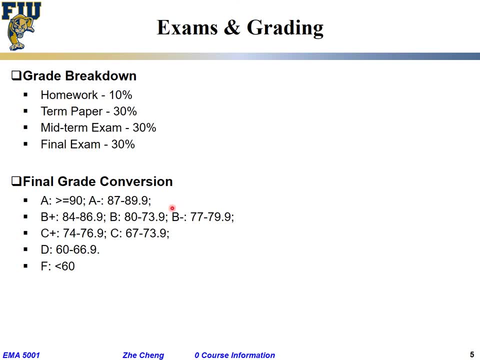 do live ă'veJapanese grades. I do our homework money, so you have those two. sometimes i give b, sometimes i give b minus. one or two occasions i give c plus. okay, just keep that in mind. you have to study hard to really understand the content.